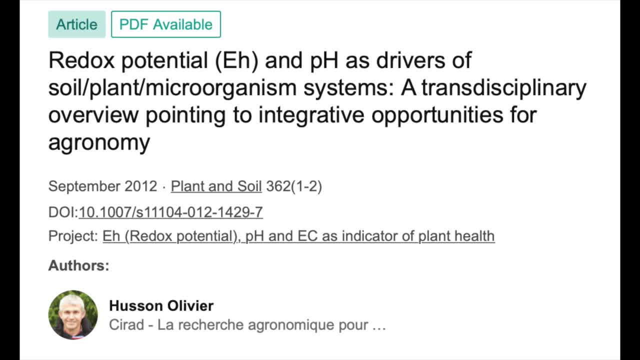 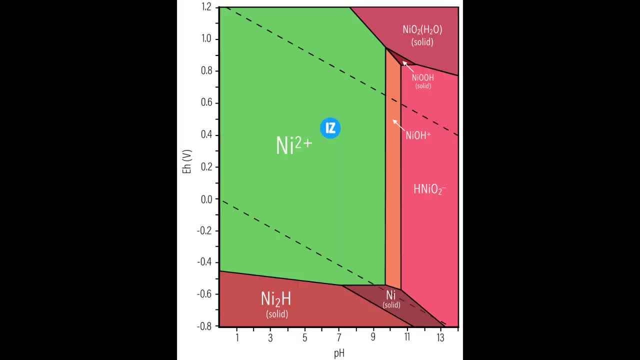 this bridge of understanding to be open to us. I'm going to be referencing a lot of my book today. I'm going to be referencing a lot of metadata, a lot of composite data from years of working with folks like Dr Olivier Roussan. 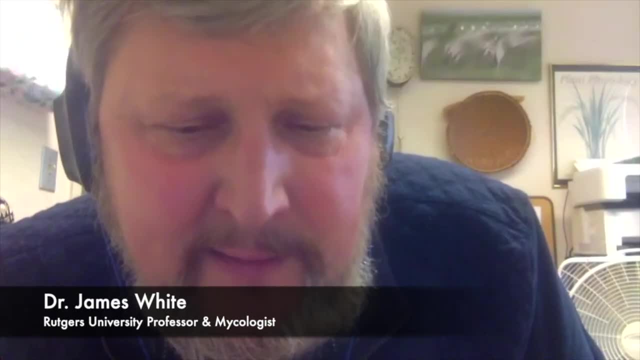 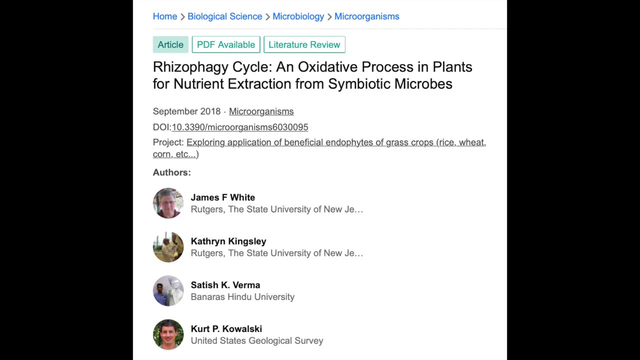 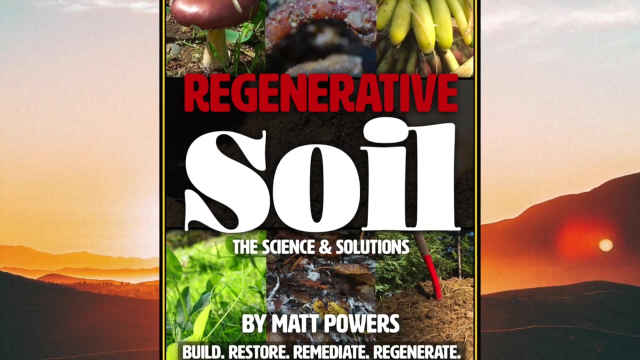 learning from people like John Kempf, as well as professors like Dr James White, who are testing everything right now in the roots, developing new stains, all of that. I am tied into all these people and learning from them and I am trying to represent them as best I. 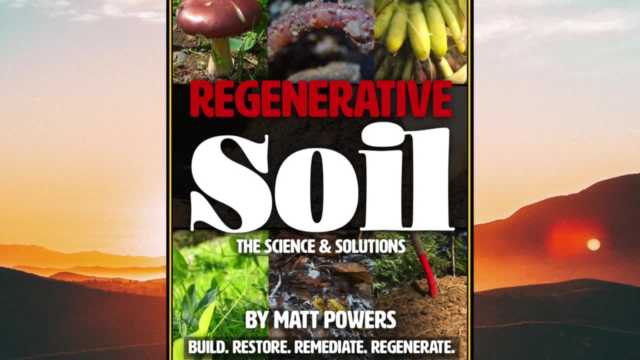 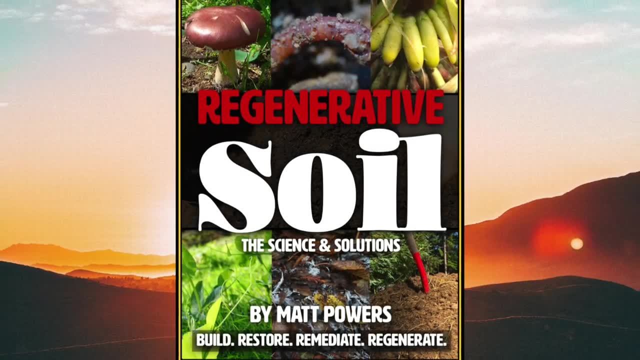 can. So, with that caveat, understanding where we're coming from, understanding that this is an introduction to a much larger concept that will affect everything: the way you see the world, the way you understand the world and interact with it. So, that being said, let's dive in. 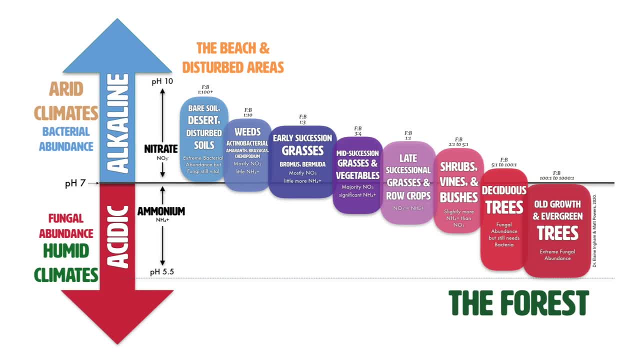 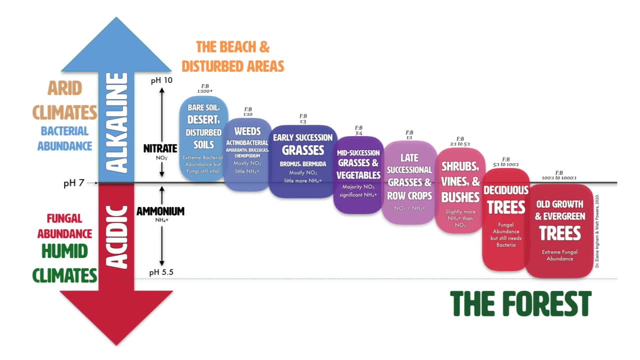 So many of you have seen this diagram in different forms. Many of you have seen the succession, the forest succession from beach to forest. Some of you have seen it related to the forest being more fungal, dominant in the beach and disturbed areas. Some of you have seen it related to the 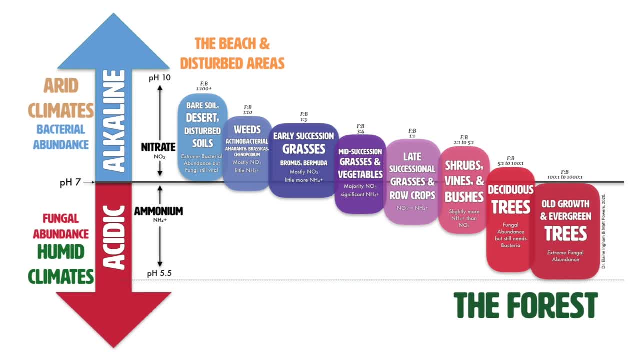 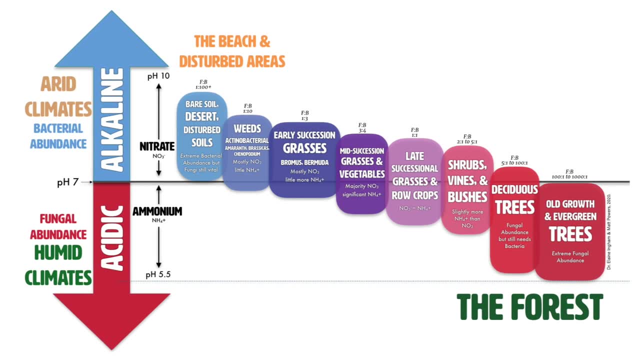 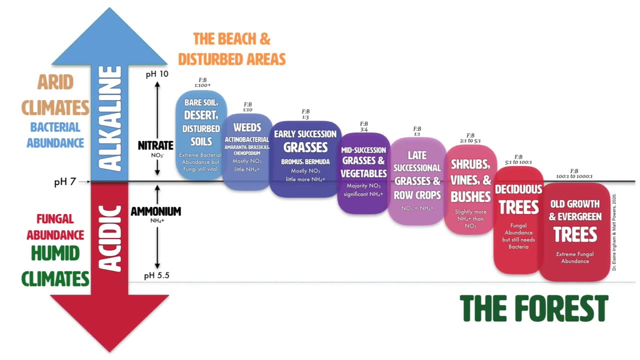 lacking in fungi. But there's some sophistication there that over time has arrived stronger and stronger, that you know. not only is it alkaline, but it's nitrate dominant And not only when it is acidic it's ammonium dominant. We realize that there's fungal abundance, ammonium and acidic. 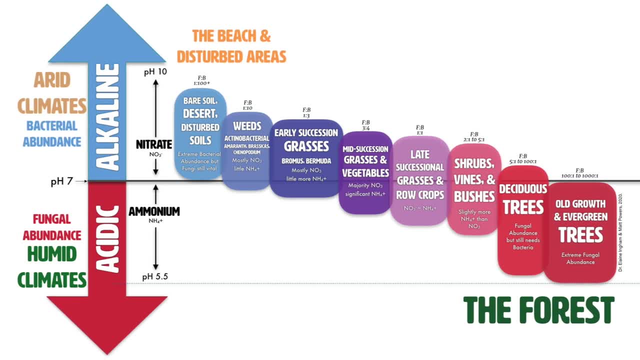 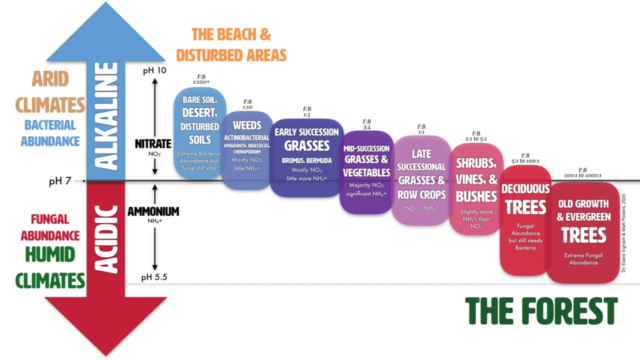 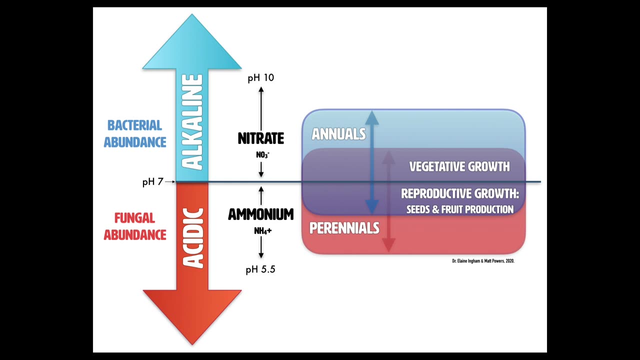 linked with humid climates. And while this is true, there is a world of complexity beyond this representation. And it is also true that annuals and perennials need an overlap, a ratio, a different ratio depending on who they are. of nitrates and ammonium, They need a swing. 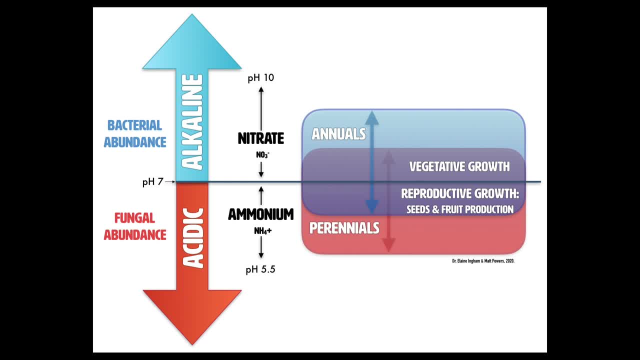 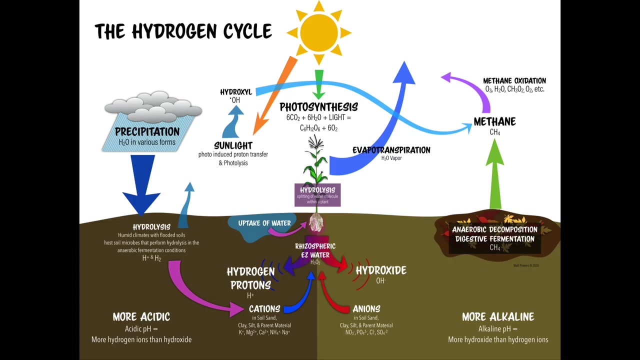 throughout the season, and they need always both. So it's not either or. but even this is not perfectly clear. There's another layer to this, okay, And I want us to look at this from the pH side at first, because pH is the power of hydrogen And because it's the power of hydrogen. 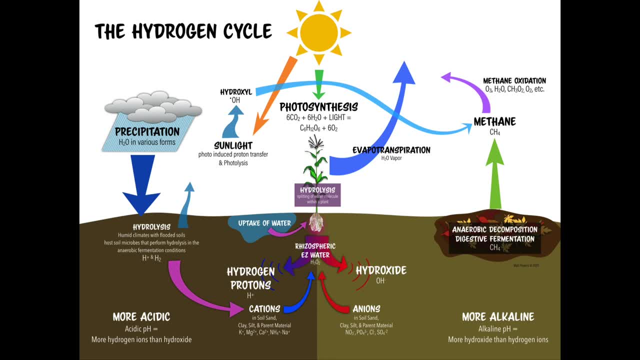 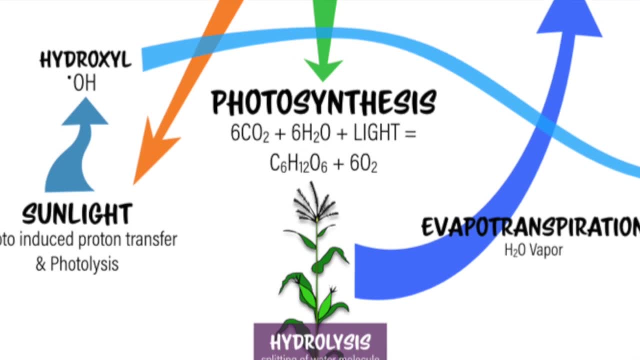 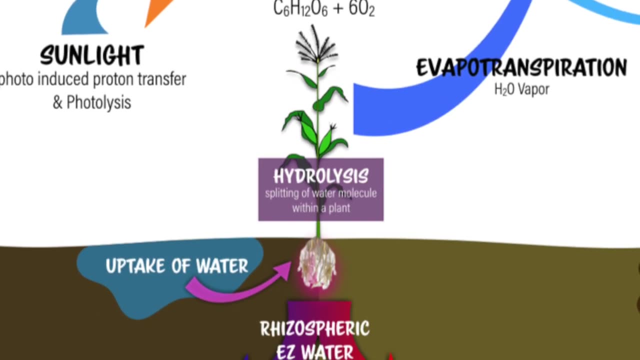 it has to do with the hydrogen cycle And it has to do with photosynthesis and the way that plants interact with the rhizosphere, the world and the root layer and the soil. They are either releasing protons, hydrogen protons, or hydroxide, So that's either H plus, which attracts cations. 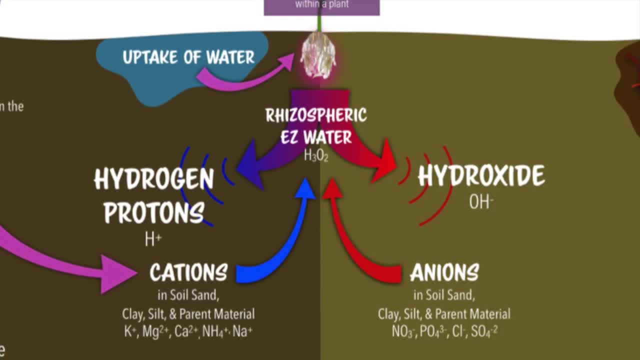 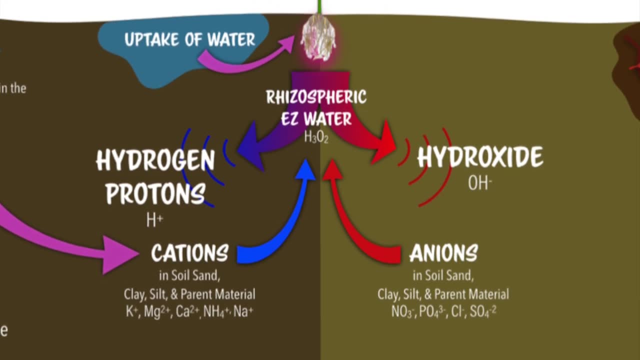 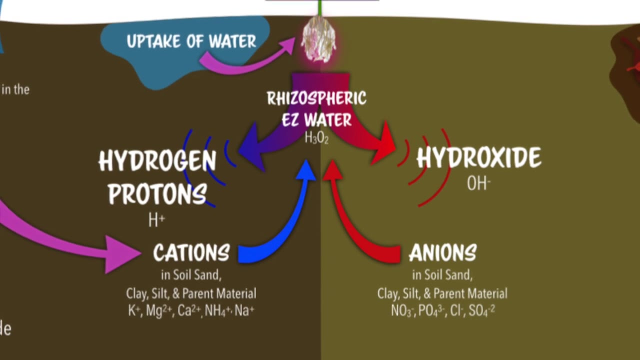 or OH negative, which attracts anions. Sound like the classic chemistry? Oh, you better believe it, because this is the seat of pH. pH is actually measuring the concentration of protons versus hydroxide in the soil. So if you are really alkaline, you have more of a chance of getting a. 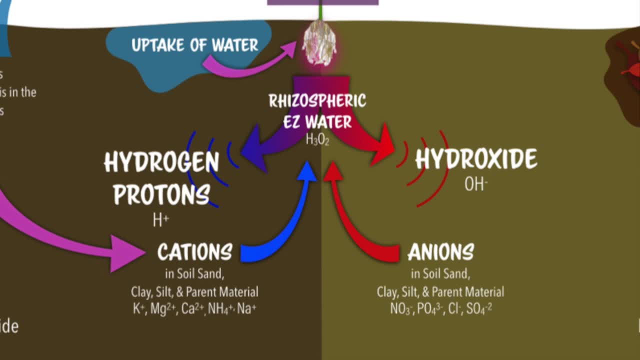 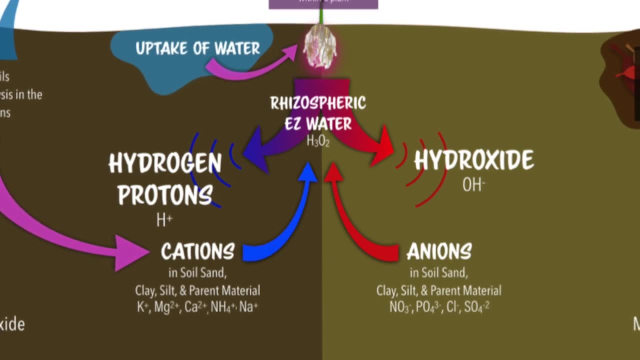 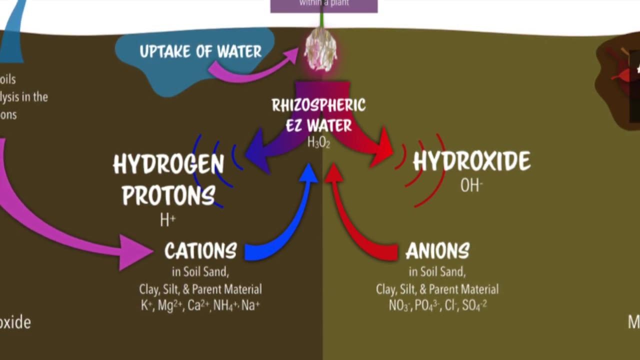 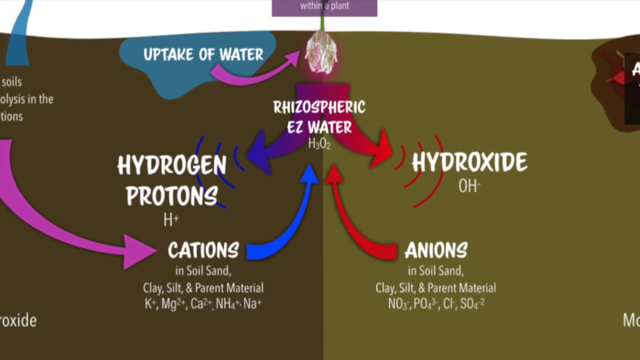 more hydroxide than protons, And the reverse is also true if you're acidic, So at pH neutral, pH seven, it's water, it's neutral. but we have to understand that it's an averaged out number. No soil that is natural is uniform in pH. It changes every micrometer, sometimes pH four to nine. 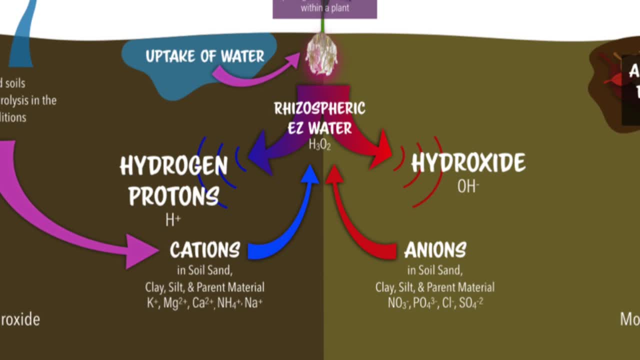 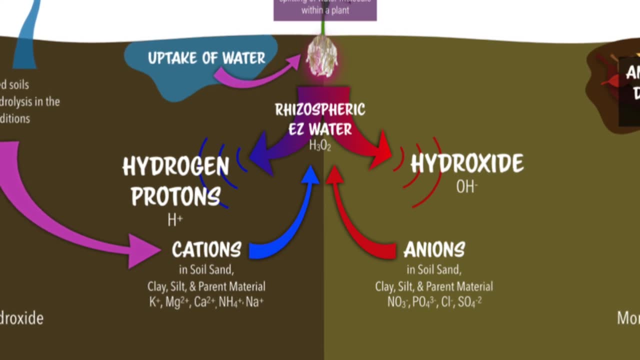 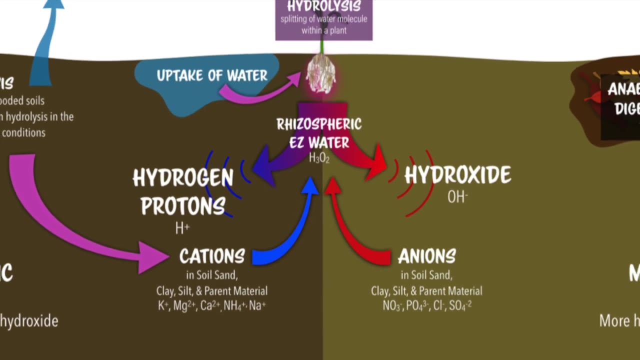 but these are averages that we're getting and the plants themselves. they're directing the direction of the acidity or alkalinity, They're determining the pH. So this is a page from my book. I go through all the diagrams of all the critical nutrients and 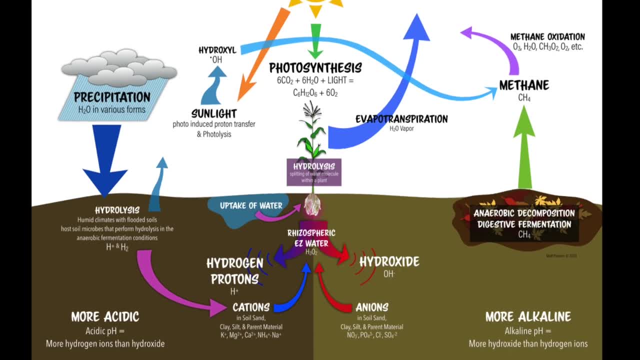 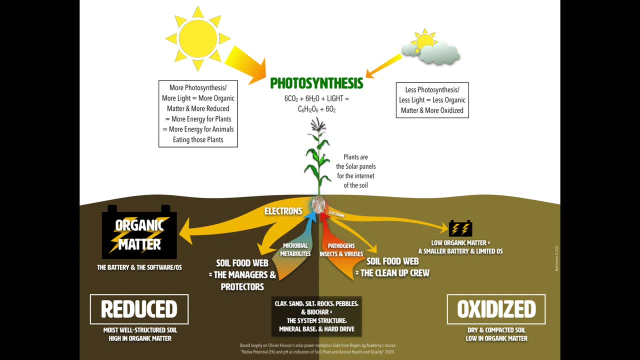 elements for plant life and that are key to soil, because plants are key to building soil. So if we look a little closer though at photosynthesis from that electron perspective, that proton perspective, we suddenly, we suddenly see a different way of measuring things, The energy that's coming in from the sun. 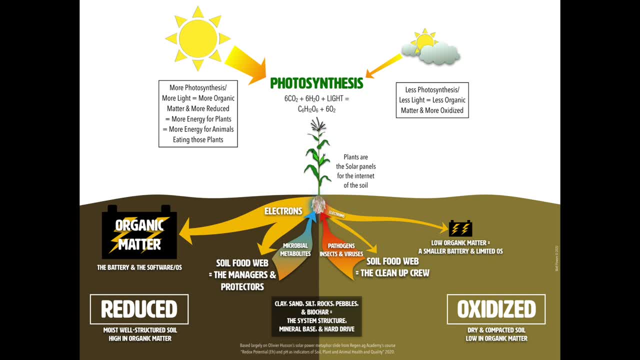 through photosynthesis gets turned into energy held in the organic matter. So the electrons actually are held in the reservoir of the organic matter in the soil, And this is why it's so important to have organic matter. And it's also true that the more organic matter you have, 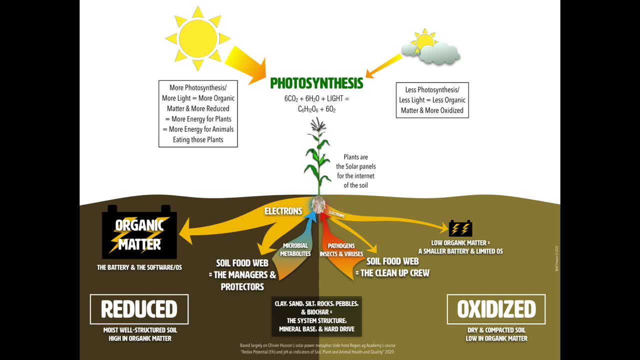 the more energy you can hold and the more you can hold, And so that's why it's so important to have organic matter, And so that's why it's so important to have organic matter. So in this case, your soil is going to be hundred percent organic matter if you have the right amount of energy. 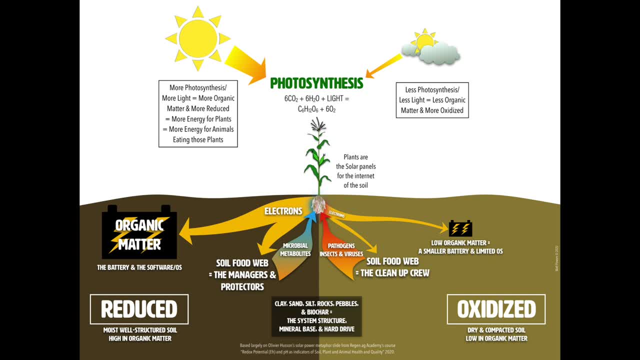 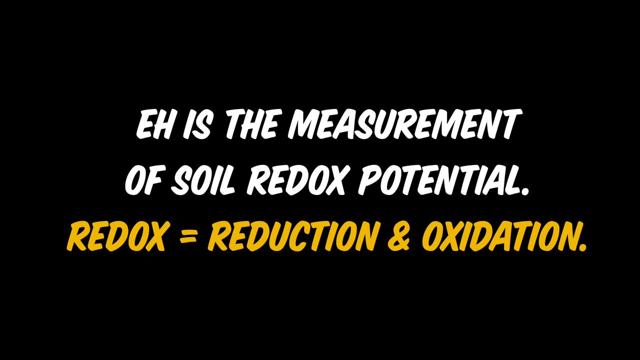 and then you can buffer your soil towards the pH EH ideal zone. So I just said a new vocabulary word there: EH, and that is what we're here to talk about today. Soil redox is EH. EH is the measurement of soil redox. potential Redox is reduction in oxidation. Now you've heard of oxidized things. 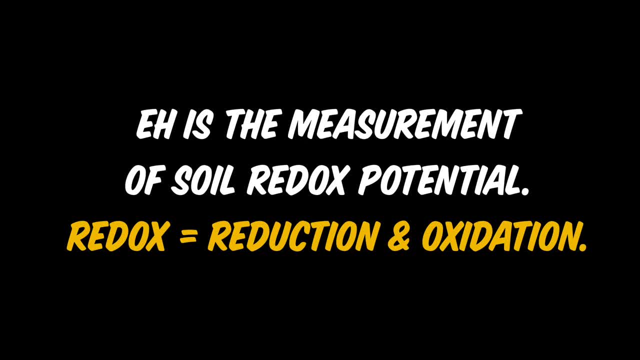 You've heard of oxidized soil, probably, but you probably haven't heard of reduced soil, because it's a chemistrionic reaction. It is a chemistrionic reaction and the point is you have to come up to a position where you've got lots of oxygen in your environment, Because it's a chemistrionic reaction And you've got lots of oxygen. 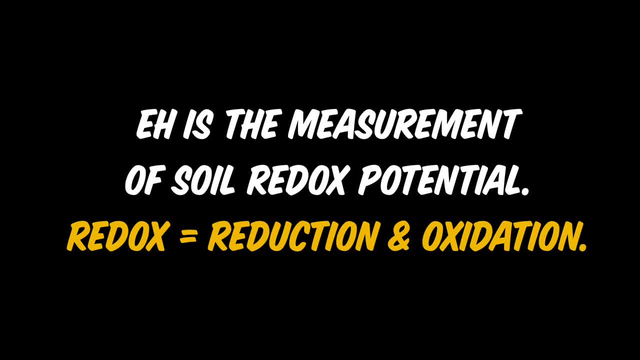 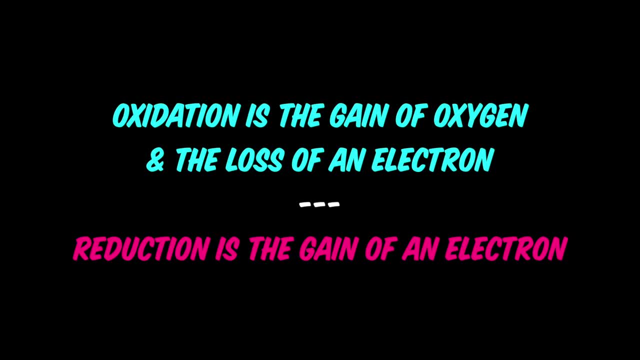 term And reduction refers to energy being added to the system. I know that sounds crazy. that we're reducing the soils mean we're adding energy to them and often increasing the soil volume and enriching the soil with nutrients, That means we're adding to it. We got to forgive the chemists. I. 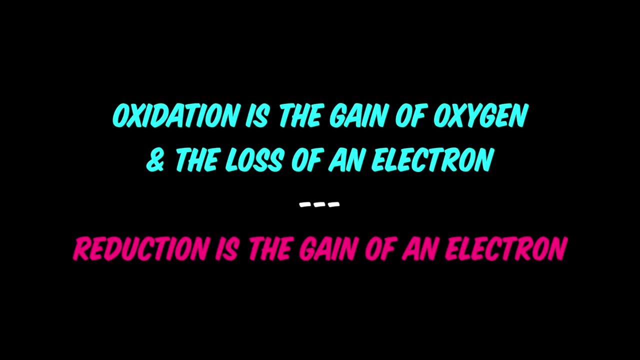 mean, when they get something wrong, they never change the name for it. They just keep going and expect everyone to memorize their mistake. Like you know, selenite doesn't even have selenium in it, for instance, And so there's no revision happening, And so we have a lot of these terms. 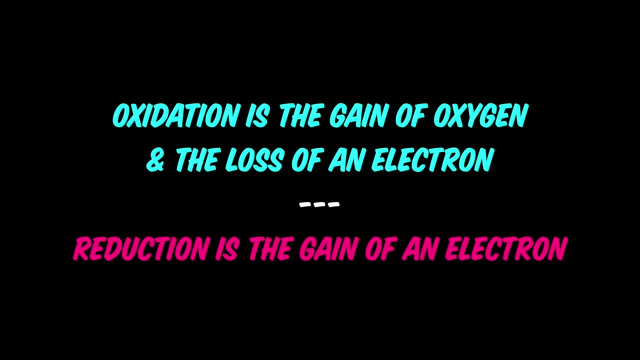 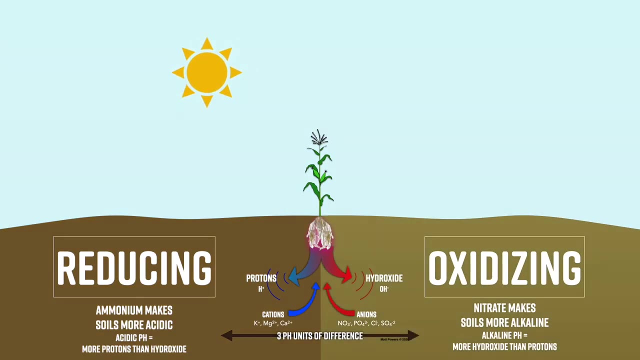 that are somewhat difficult until we memorize them. Reduction is one of them. So redox is reduction in oxidation. It is a scale like pH, like H plus versus hydroxide, Right? So let's just look at that right here What that looks like. This is an animation. Just take that in. 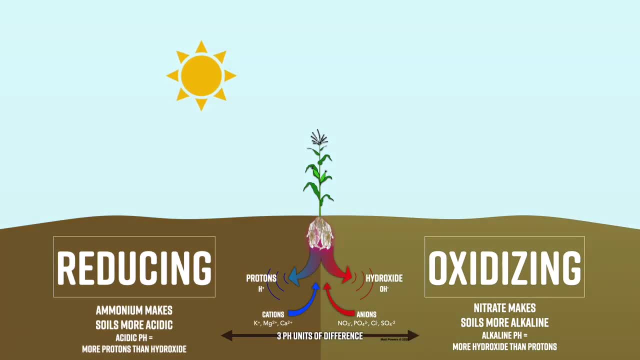 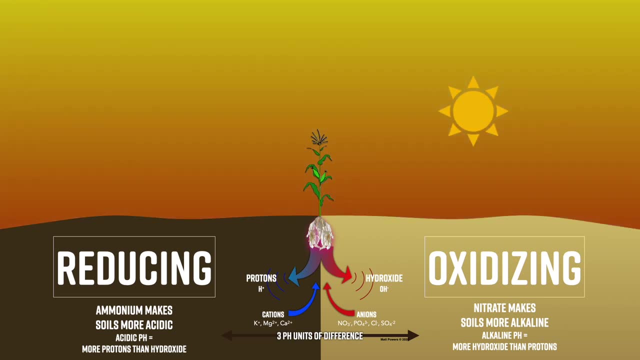 for a second. I'll play it again. You can see that where it's where it's able to reduce, it's getting good sun. It makes the soil darker. It enriches the soil, adds energy to the soil. where it's oxidizing, It's harming the soil. 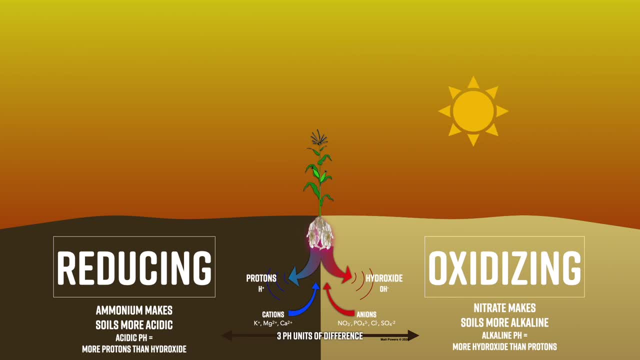 and making it lighter and there's less sunlight, So it's actually a combination of things that can oxidize the soil. It's not just the soil, the plant stress. It could be that there's not enough light. It could be photosynthesis related. 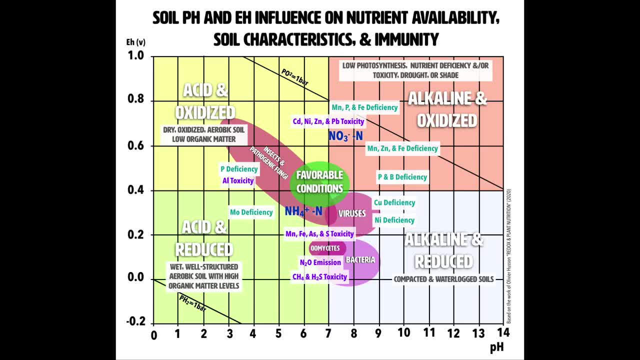 This is a chart based off the work of Olivia Huson in the Redox and Plant Nutrition 2020 published paper. He is absolutely amazing in the work that he's been able to accomplish and amazing as a person- very open, very willing to share and discuss and teach, And this chart really shows. 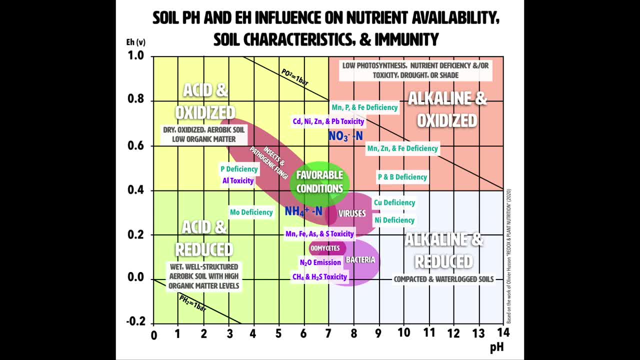 you where the favorable conditions are and and also shows you where we've gone wrong. So if we look at the bottom left, acid and reduced, that's wet, well-structured aerobic soil with high organic matter levels. And then we look up to the top right, alkaline oxidized, that's low photosynthesis nutrient. 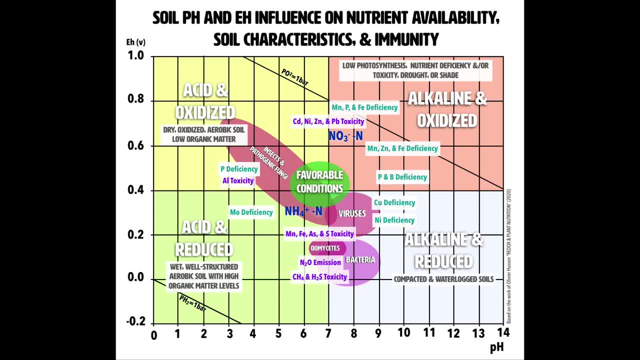 deficiency and toxicity, or drought or shade, And this is actually where the beach and disturbance is. this alkaline oxidized And the acid and reduced is where the forests are And if you go too far it becomes the peat bog. Right, right, right Makes sense. 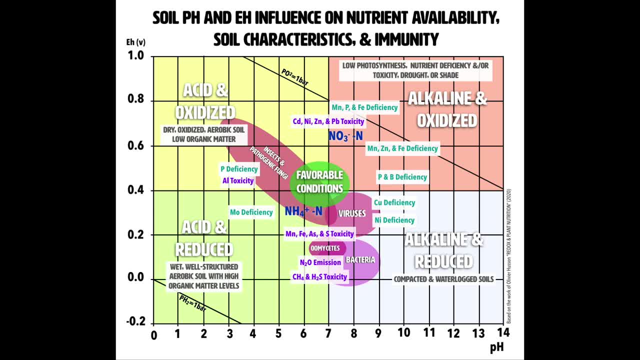 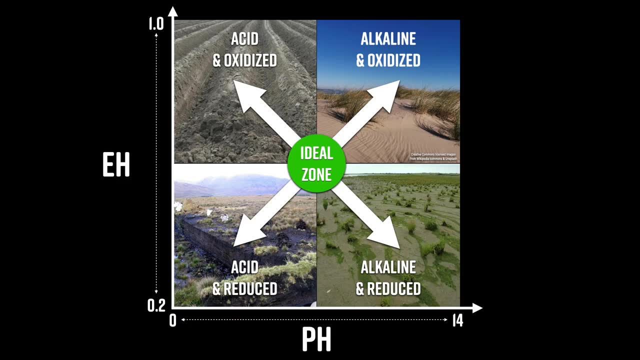 So what are the other two corners? Well, let's look at it like this: If you're in Montana and the soil's chemistry, the soil chemistry is leaning towards acidic- the actual minerals. when you tell it, you've oxidized it by combining it with air. 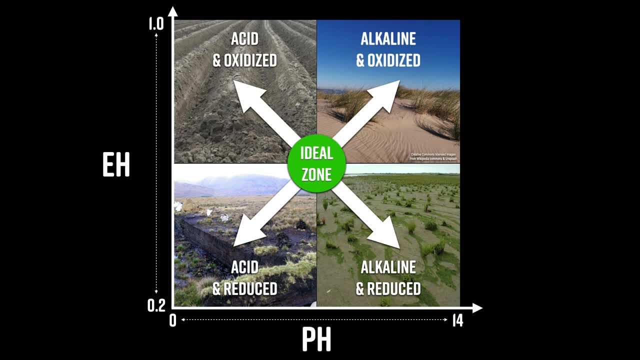 So that is acidic, Oxidized soil, And then alkaline and reduced. well, that's waterlogged soil and it's alkaline. So that that's, you know, the salt marshes. That's like that crossover area between the ocean and the land. 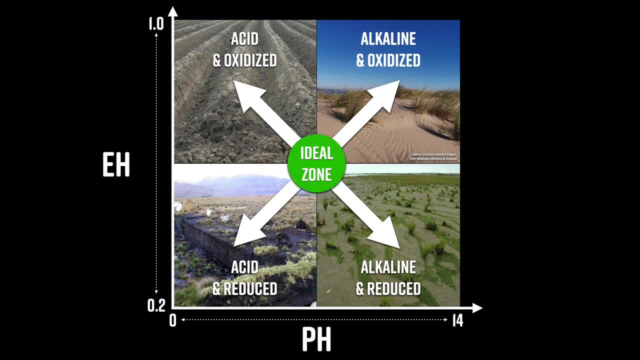 So it's dry on top, It's wet on bottom And it And so we suddenly see that we need a little bit of all these places a degree. We need it to be a little bit dry, We don't want it too wet. 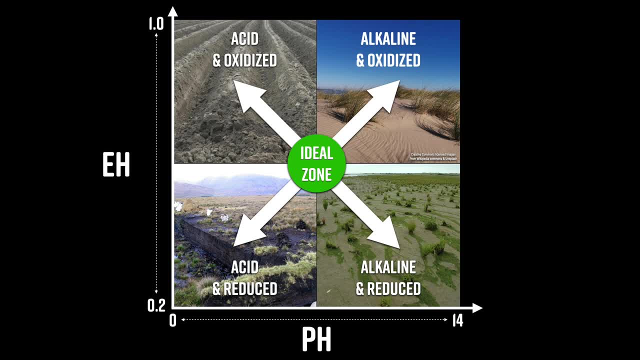 So so we want some compaction, We want some aeration, We want some alkalinity, We want some acidity, We want some energy, We want some cations, We want some anions. So the ideal zone actually allows the plants to easily direct with the minerals. 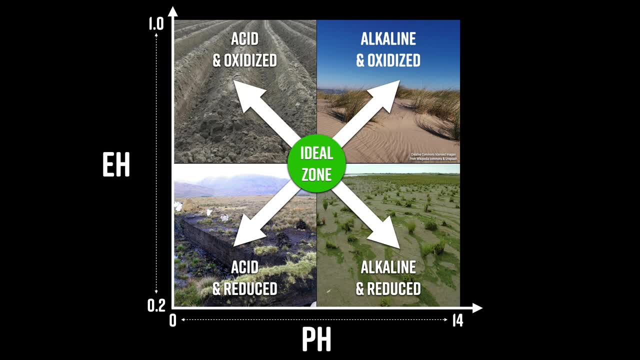 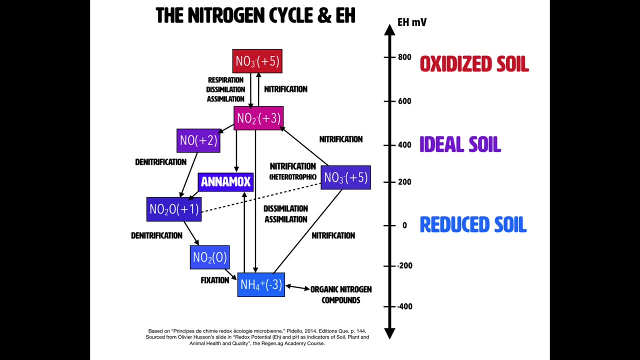 And so that's what we're looking at here- is the minimal amount of energy, The direction that's happening at that root zone layer and usually at that individual root hair, because once they start a conversation they tailor it to that microbe. And if we look at just the nitrogen cycle, we see that different forms of nitrogen are available at different levels of oxidation versus reduction. 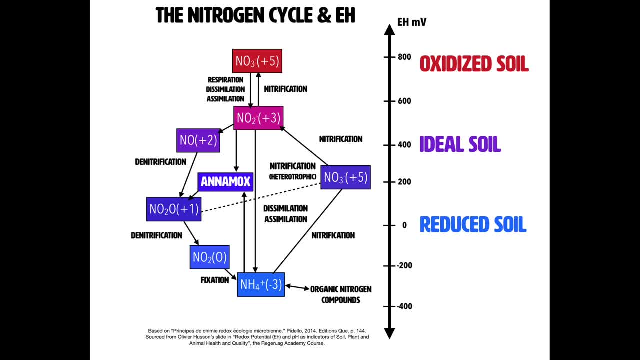 And, if you think about it, when it rains, water logs the soil, you have a pH and EH effect happening right there and then, which unlocks things and locks other things out, no doubt, But these things are happening fluidly all around us. 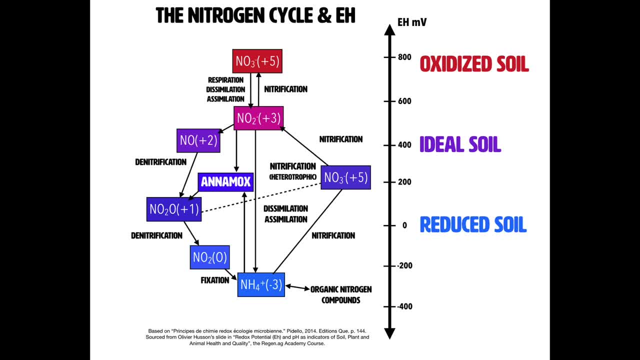 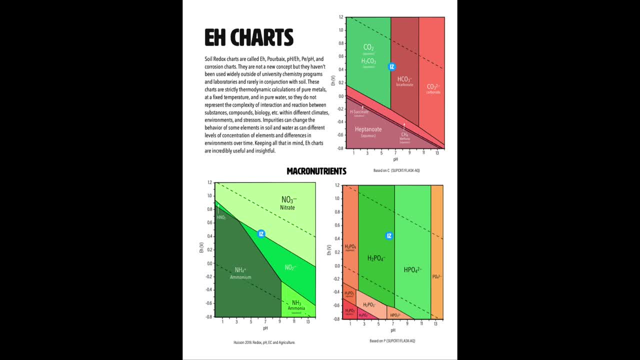 And also the microbiology has the greatest control over this. So they're doing it too. These EH charts, or Paul Bayes charts, or pH charts, They're not going to change. They're not going to change. But these pH, EH charts, or even PE pH charts, they are chemistry's classic corrosion charts for every element. 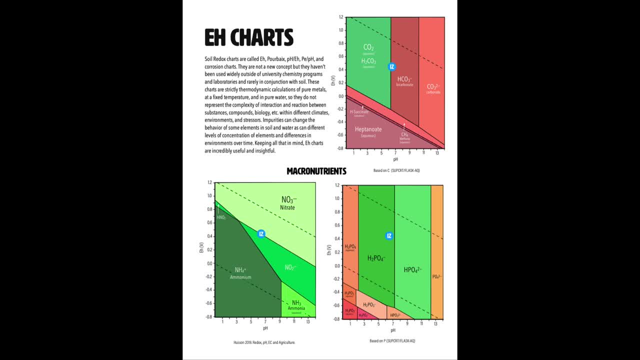 I want you to take that. in classic chemistry, of course, is thought about which elements are stable in which states. This is just what they do. This is you know, but it is also purified chemistry. There's no other elements interacting usually in this, unless they put them in there. 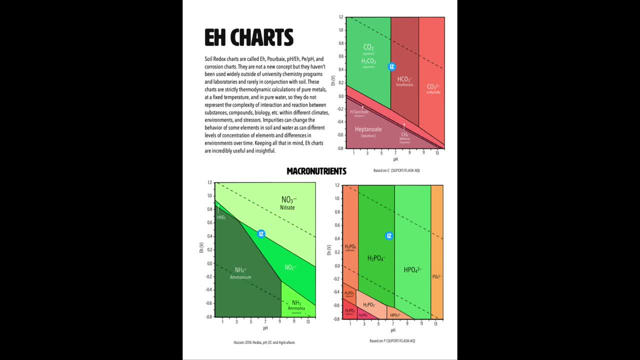 So these are mathematically calculated and created. This is, they put in the different elements to interact and create the charts. That's why some of these charts are composites of several charts, So they include all the different elements in the testing process. 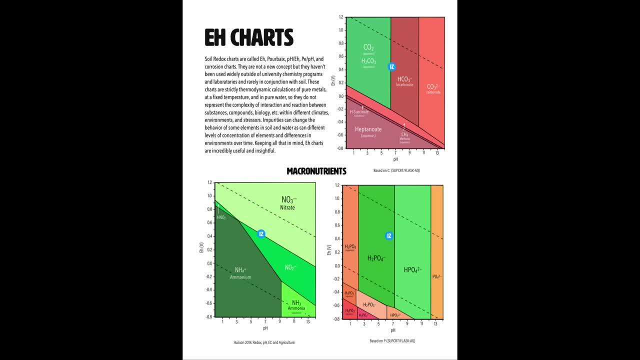 And then so these are talked about. There's lots of different ones online, depending on what elements they're feeding into the data set, And I've chosen these for the soil data sets. I've chosen these and color-coded them myself to show what's green is good, what's red is bad. 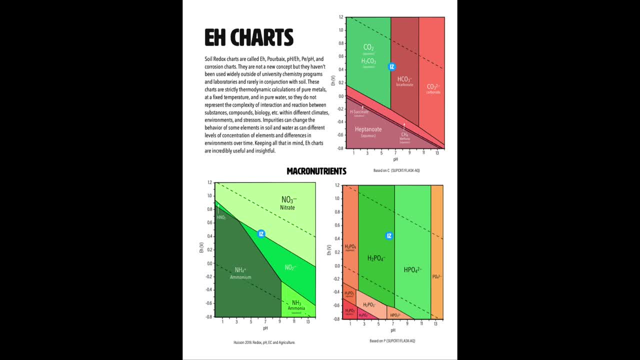 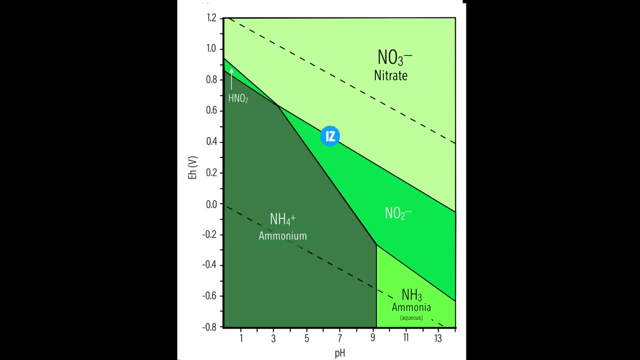 So we show toxicity, So we show the macronutrient and micronutrient availability And we also seek the complexity, right. And when we look at nitrogen we suddenly see, wow, Nitrogen has been so complex. Wow, Sometimes your pH seems to be just perfect. 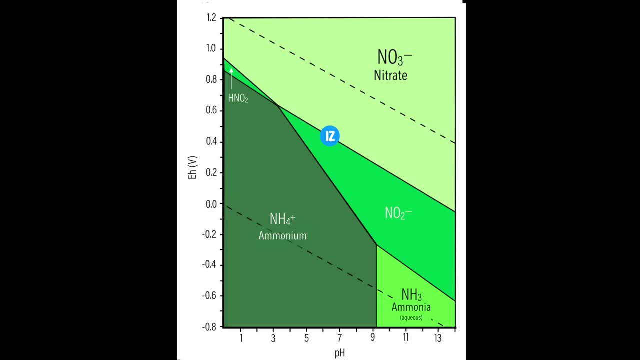 But maybe you just tilled, Or maybe it just rained too hard And now you've got the EH bouncing up and down, And I mean, the pH is bouncing up and down too at that time too. But the EH may be something that you aren't thinking about. 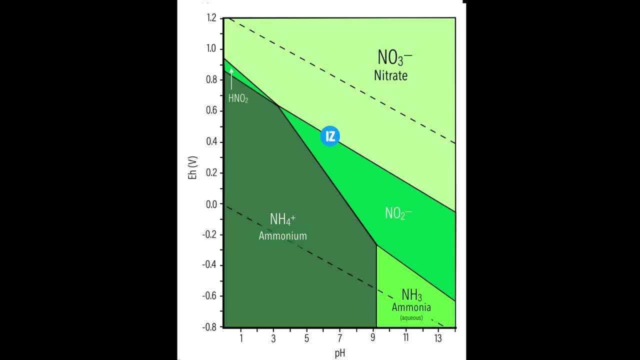 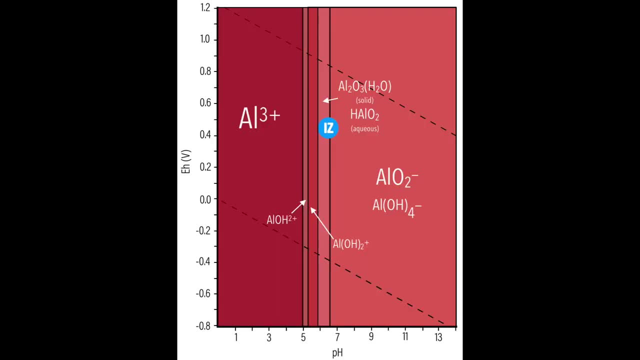 And that's the reason why that form of nitrogen Nitrogen isn't there And you know some of these things do operate along pH. I know that some toxic things like aluminum we always talk about- oh, you don't want, you know, to get into this range. 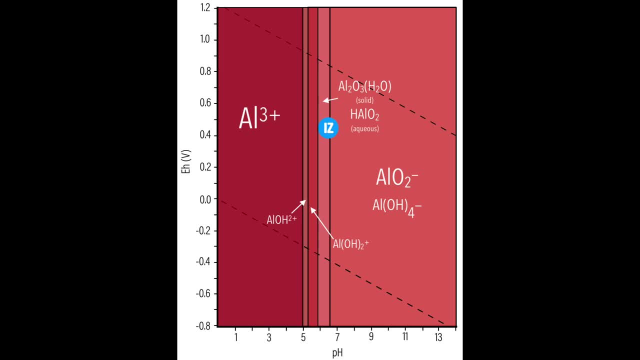 But hey, look, there's an aqueous form too, And we know that some plants have no mycorrhizal filter to protect them, So they could be taking it up there too. So we have to really look at these things from a scientific perspective and go through and, yeah, understand, like. 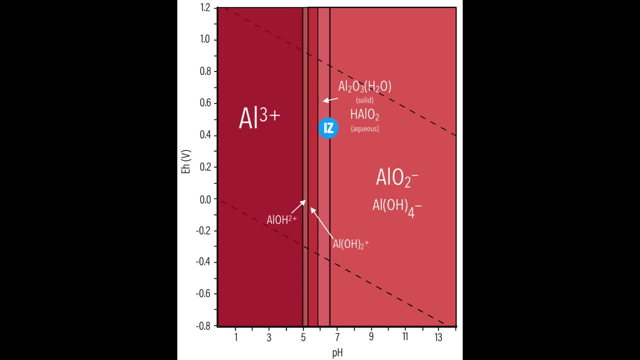 as a cation, it's released acidically, But if it's already in aqueous form, there could be trouble too. So we have to be really smart with how we talk about these things And also, you know, a lot of these things are pretty darn simple. 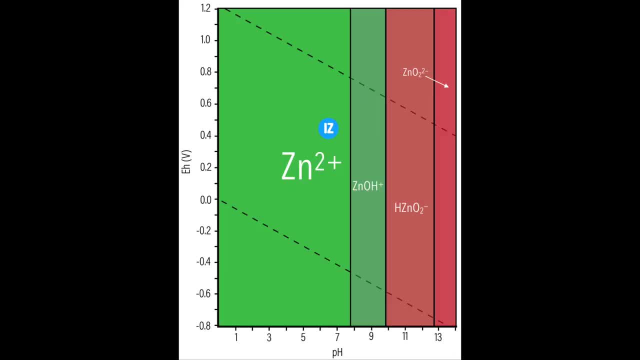 Look at zinc. I mean that cation is ready and available up to almost pH 8,, right Right before it gets oxidized, And then it's alkaline In the alkaline territory, And so we're seeing this overlap between alkaline and oxidized- I hope, because it's everywhere. 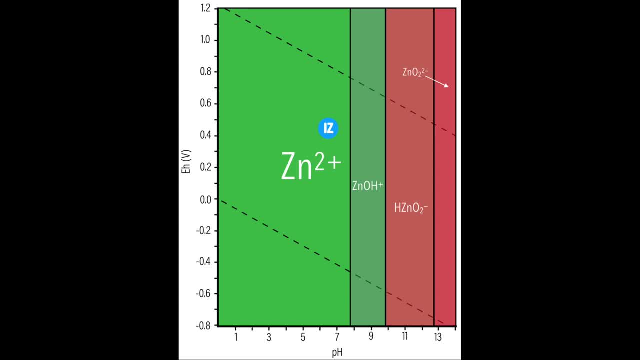 These two are partnered up and interrelated. And when we think about potassium, oh man, this is why it's a macronutrient, In evolutionarily speaking terms. we were looking at an element that plants couldn't avoid, They couldn't get rid of. 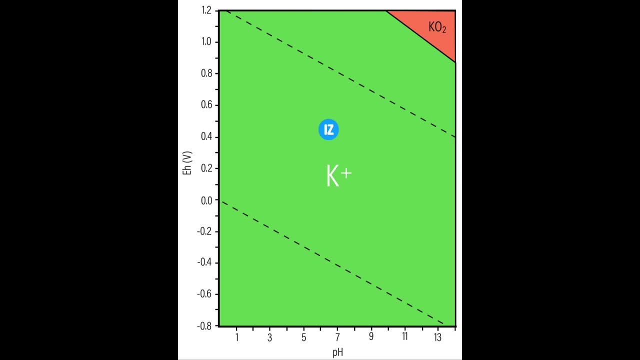 It was all up in their grill And they just had to deal with it and use it somehow. So this is very important for us to see this deeper picture, I believe, to really understand plants and soil. And that's why I've color-coded it, made it easy, made it into animations and fun things like that, so people really get it. 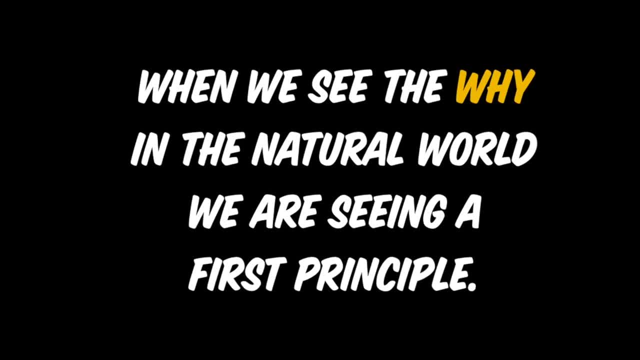 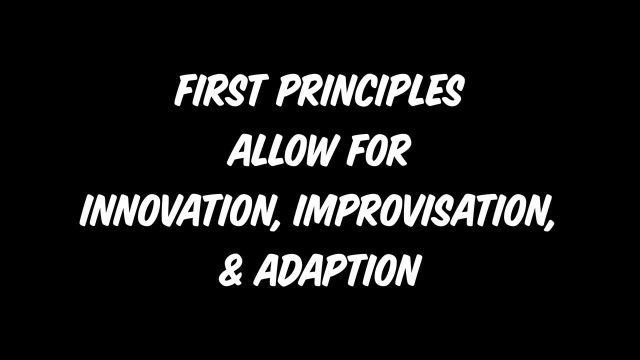 When we see the why in the natural world, we are seeing a first principle, And first principles allow us to innovate, to improvise and adapt, which is pivot power, right, But it's also how nature works. So we're being natural when we do these things. 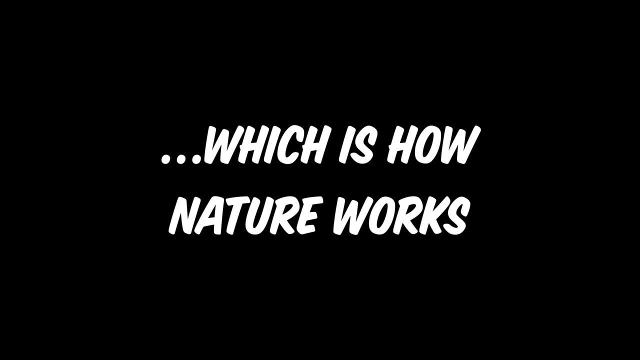 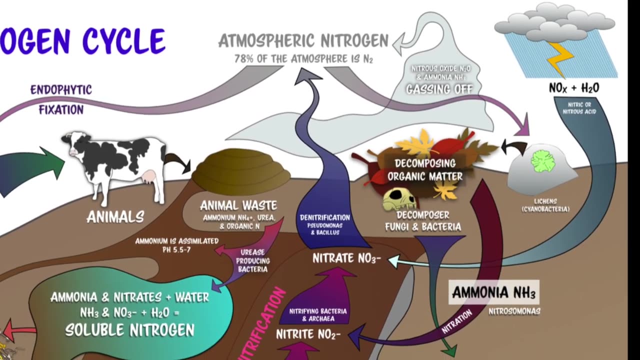 And nature is complex. but nature, I believe, is understandable. And when you take the actual, which is what I did for all the cycles as well, I don't have just the corrosion charts up there, I actually mapped it into the reality to show the micro to macro interconnections and pathways for everything. 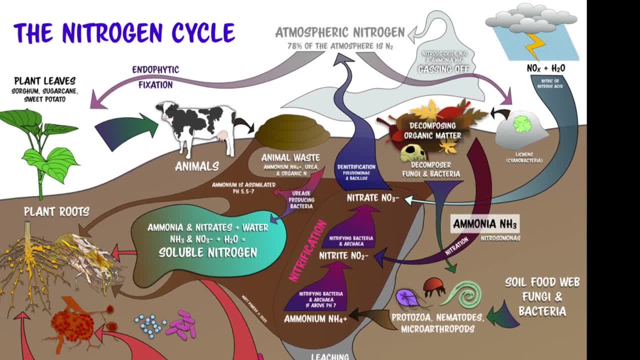 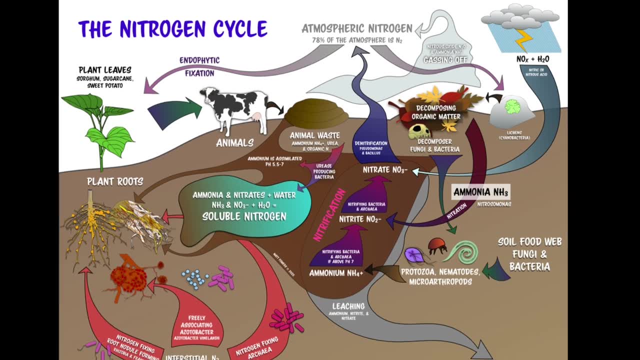 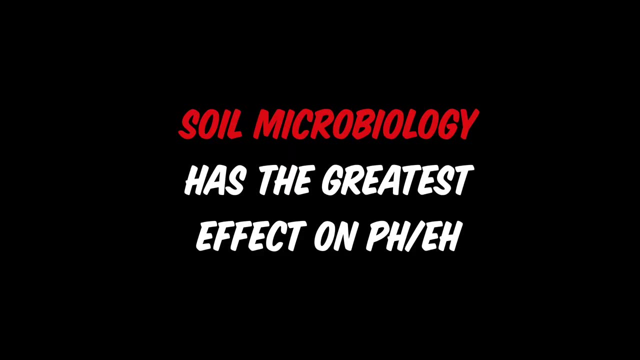 Every soil plant nutrient, all the essential ones, even the essential trace ones that are sometimes controversial. I even delve into those because we have to understand that there are reasons why people are saying that they are essential. So the most important thing to take away from this all is: the soil microbiology has the greatest effect on PHEH. 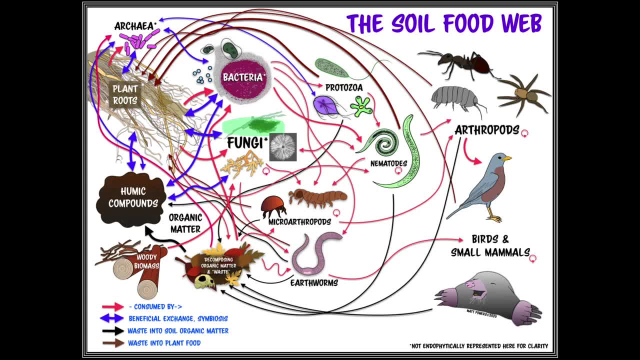 So the soil food web. going back to my soil mentor, Dr Elaine, I've learned from her one-on-one throughout the process of writing all of my books, as she's personally reviewed and discussed these things and actually helped her as well in some of her stuff. 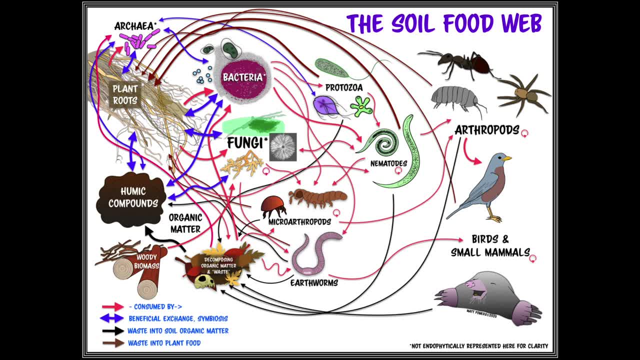 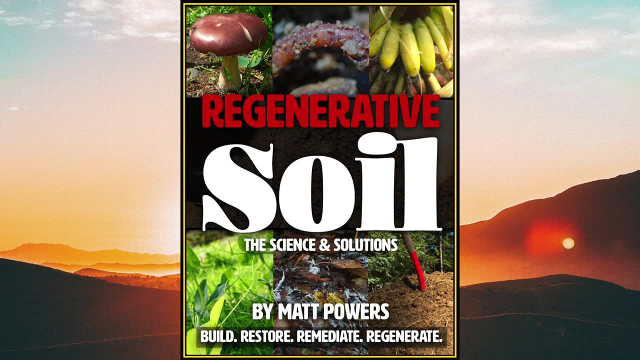 And so I feel so much respect and deep value for her introducing the soil food web. This is all part of the new course Regenerative Soil and part of my book Regenerative Soil. Regenerative Soil, which has been called my best book so far, is being used and recommended for everyone by David Holmgren, the co-creator of Permaculture. 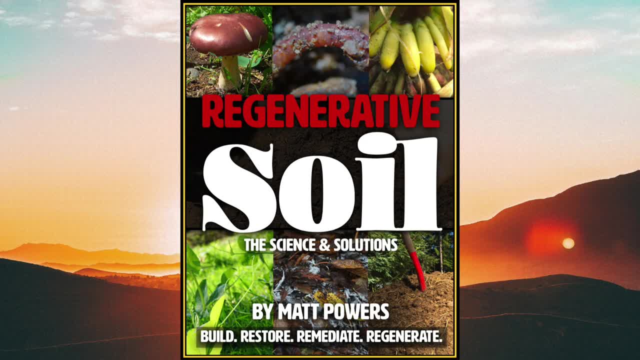 You know what I mean. Talk about influences, Talk about how all this has been a culmination of all my studies. I've been able to combine and find the first principles in creating natural farming in the biological farming Dr Elaine Ingham world. 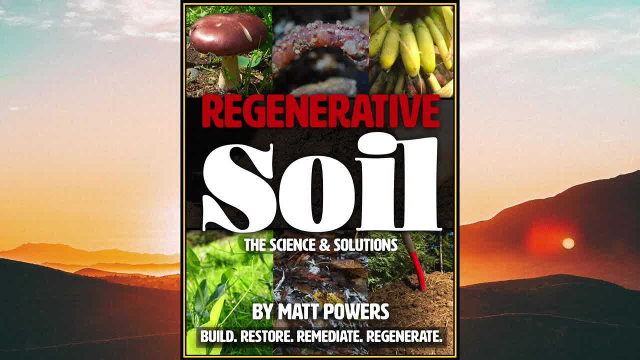 In the jungle, In the non-Kemp world, and see how they all relate. whether it's rhizophagy, whether it's mycorrhizal, whether it's the biofertilizer world, There's an underpinning language and connection between why all these things work and why certain practices in the past have harmed us so badly that we all can understand, communicate and finally see eye to eye on all these things. There's an underpinning language and connection between why all these things work and why certain practices in the past have harmed us so badly, that we all can understand, communicate and finally see eye to eye on all these things So we can make a better world. 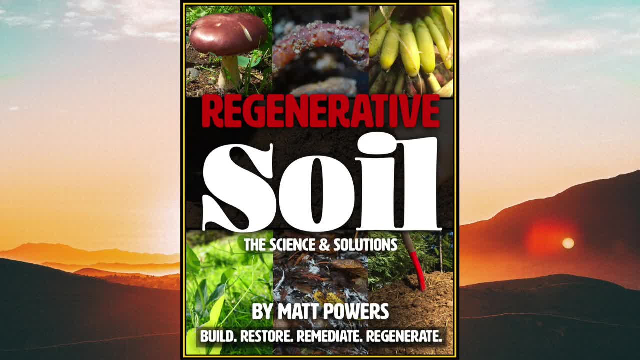 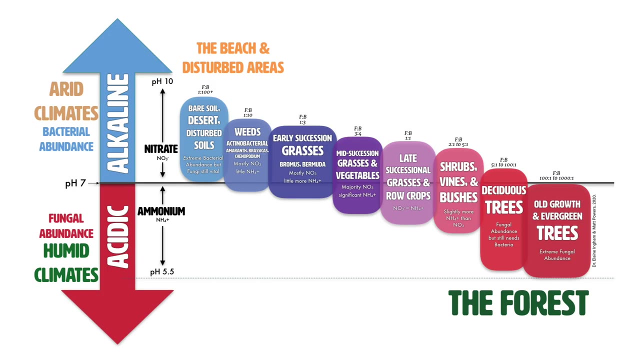 And soil redox is a fundamental linchpin and key to that conversation: collaboration, conversion and liberation from a limited way of seeing the world. I value the water cycle, I value the hydrogen cycle, I value pH, But we have to remember that it's an average we're taking of our soil. 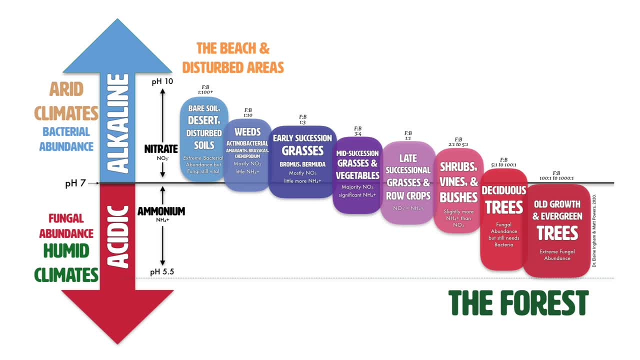 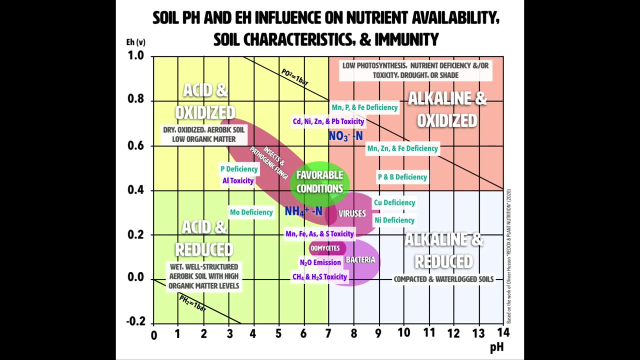 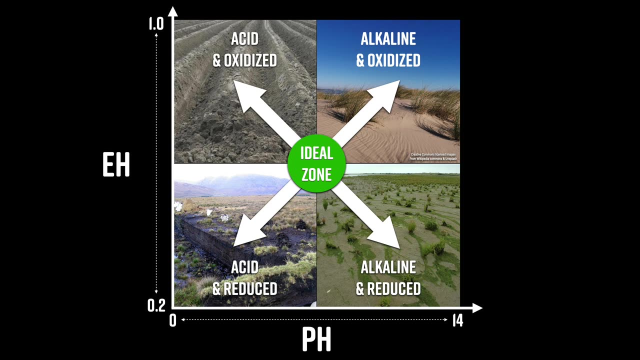 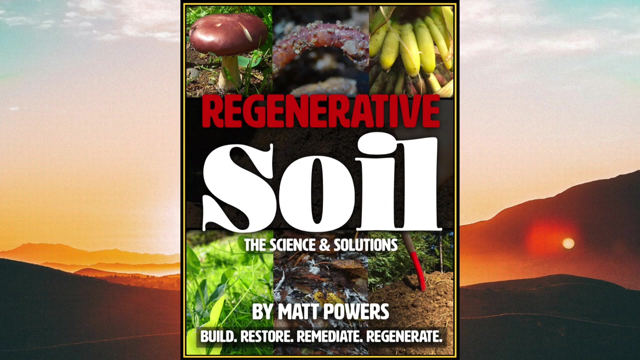 That things change at the micrometer level. We have to also remember that there's EH And even if we can't test for EH, we can go out there and do a bit of observation and quickly figure out generally what our EH is, so that we can shift it or we can diagnose a problem that we're facing much, much easier. 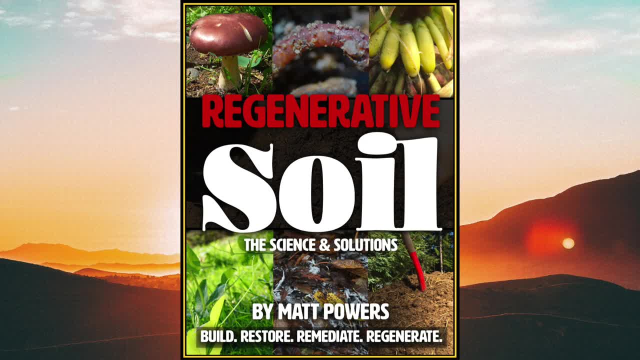 I alluded to a lot of things like how soil organicism, I alluded to how organic matter is a buffer, how EH affects food, how EH is playing out in our body, in our blood. It is literally everywhere And it's fundamental to understanding our health, micro to macro, plant, animal, all of it. 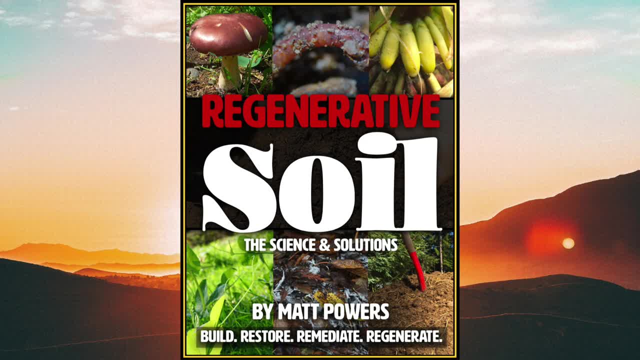 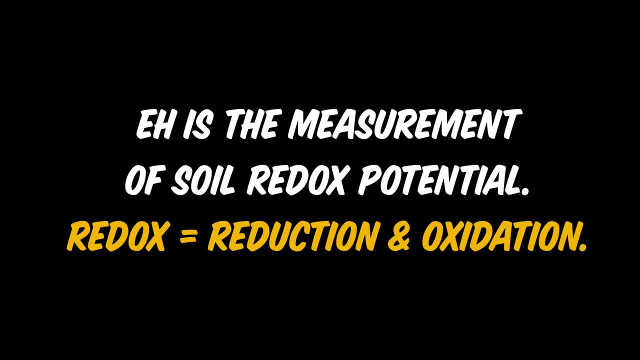 And so it's a very exciting time to be talking about this. Remember that it's reduction, redox And oxidation is the law- Loss of nutrients. So we're talking about antioxidant foods. We've just opened a whole different door And we're opening and walking into a new world together. 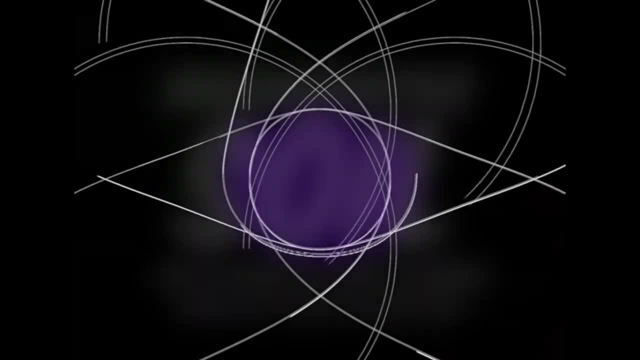 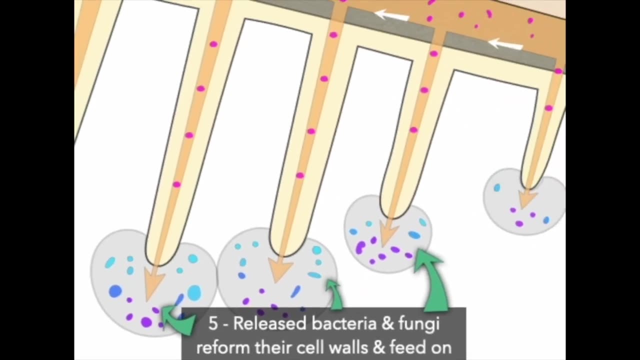 That's what this whole regenerative soil course is all about. That's what that new paradigm around soil science free webinar- that's down below, The link is below- is all about as well, Because we are about to unlock new health, new nutrition. 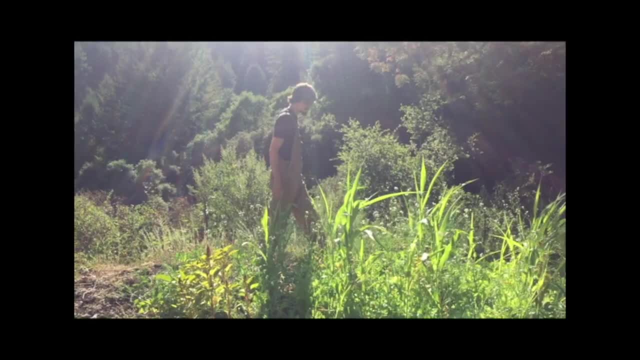 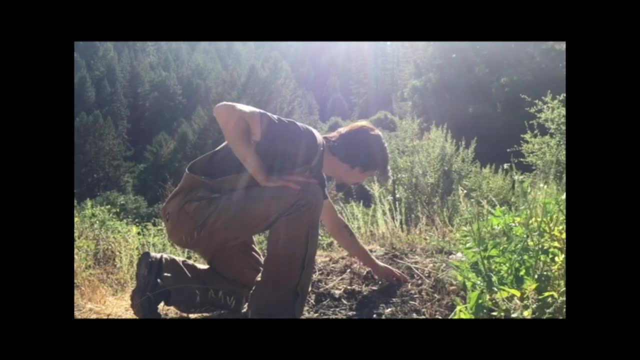 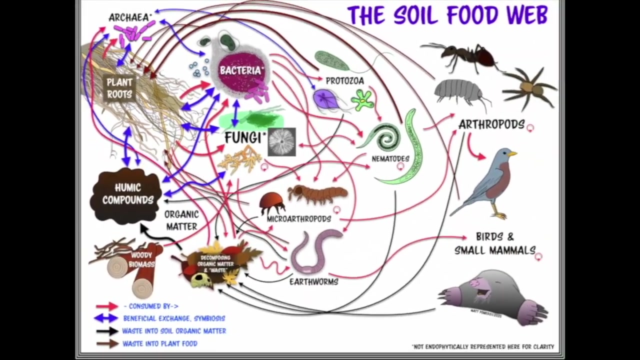 And a completely new relationship with nature, And I want you guys to be part of it. So check out the free webinar, Check out the new book. It's. it hit number seven on the on the charts on Amazon. At one point it qualifies as a best seller. 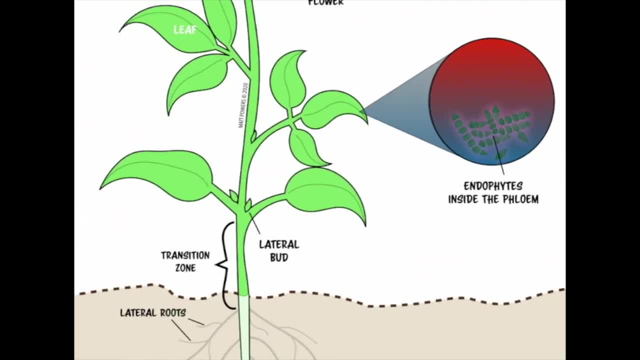 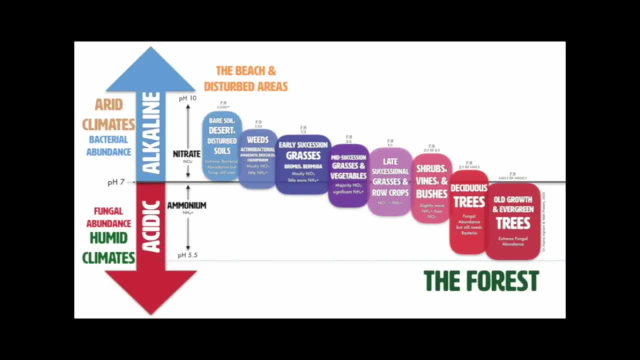 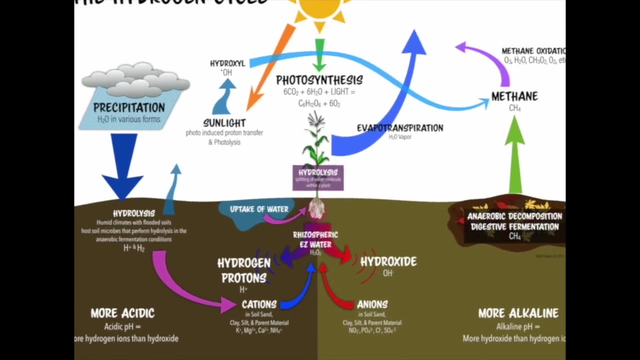 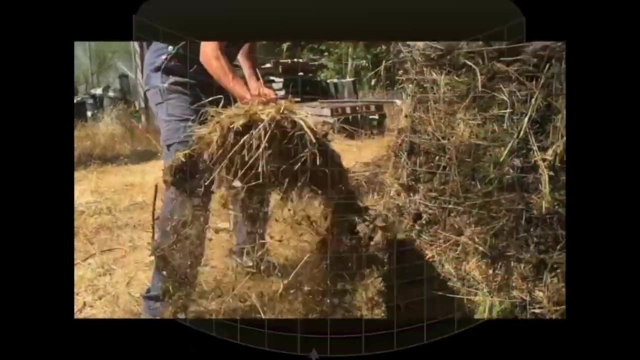 It's the most unbelievable thing that's ever happened to me as an author. I mean, I just feel intensely honored by what has happened, And It's because the information is so powerful and potent And I am a teacher and I've just been been very blessed to be in the position that I can filter these things and break them down into high school level language and easy to understand images and animations. 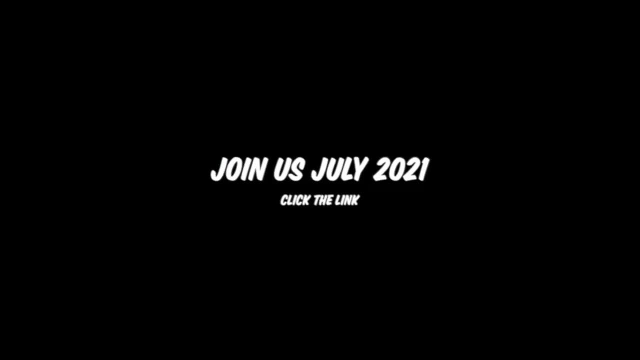 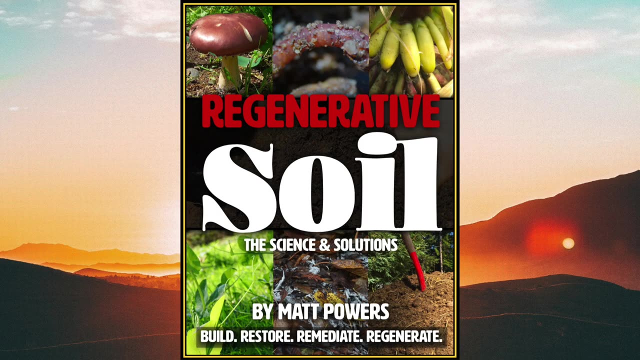 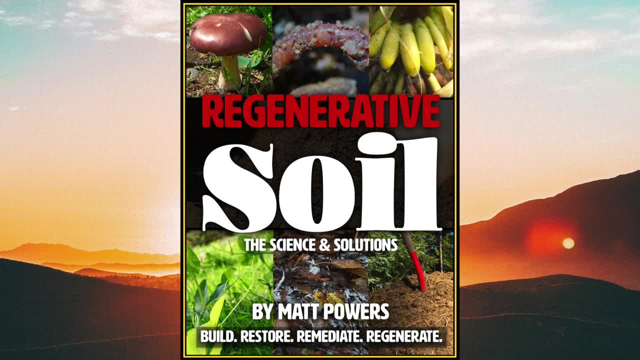 Because they are the key to the health of the planet, to water retention, to nutrients, to the health of our bodies and the future of all life on Earth. If you feel moved by this, if you feel called by this, I invite you to join me in regenerative soil. 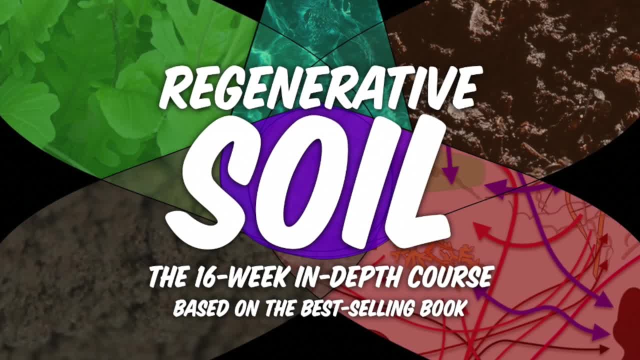 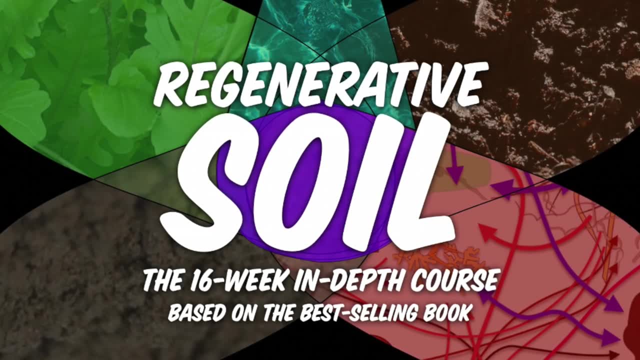 This course will change your life. It will change the way you see the world around you. If you thought this Video was was was lid flipping, please click the link below: sign up. join us for the webinars that lead up to the full course.